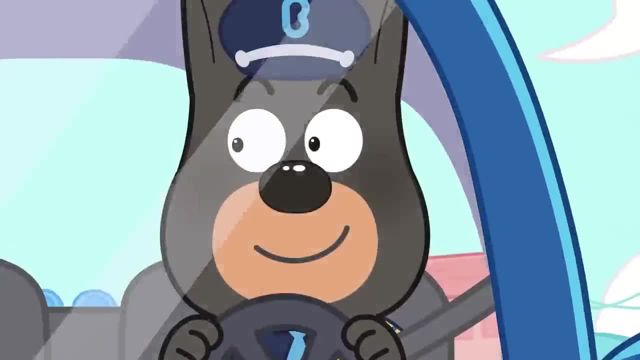 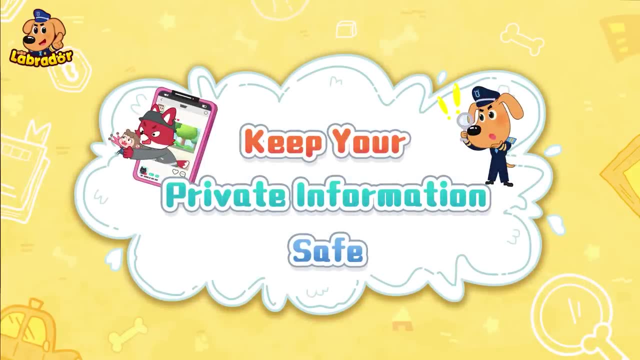 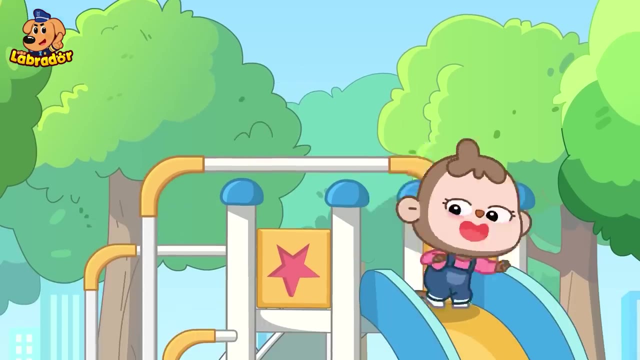 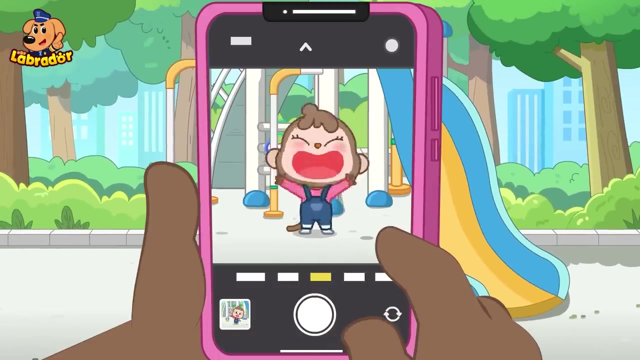 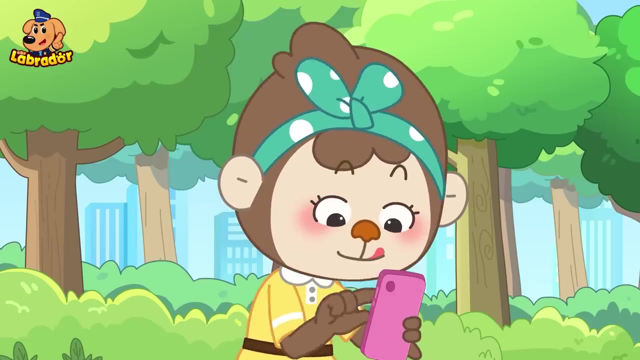 Go, go, go go. Let's go. Sherry Labrador, Keep your private information safe. Hi, Sweetie, look over here. Wow, how adorable. Well, I'm going to post it online right now. Okay, we'll get a lot of likes, right. 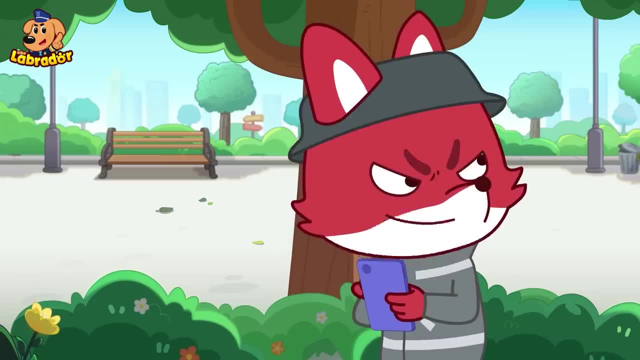 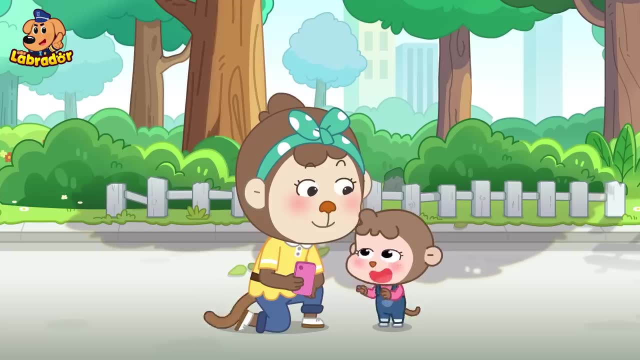 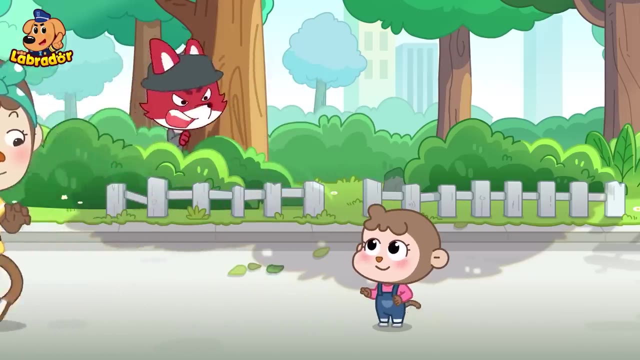 A new picture. She loves to share her pictures on the internet. It's so easy to get their information. Mommy, I want a donut. All right, Mommy, will get some for you. Wait here, okay, Okay, Finally, now's my chance. 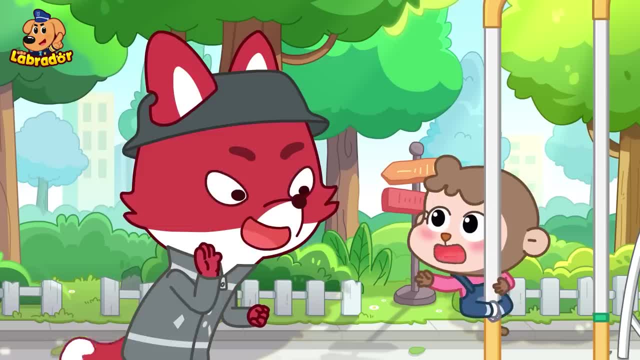 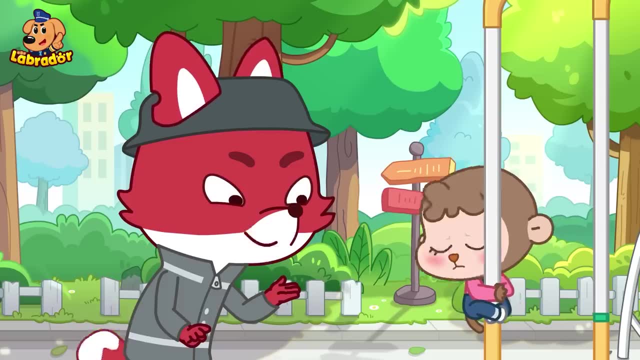 Hello, little monkey. Who are you? I'm your mommy's friend. She asked me to take you over there, But I don't know you. Your mommy told me a lot about you. You're four years old and go to Sunflower Kindergarten, right? 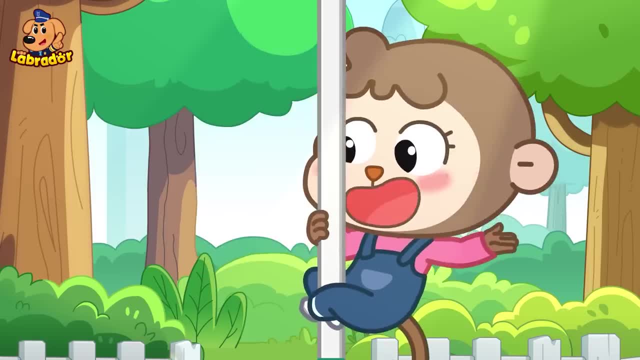 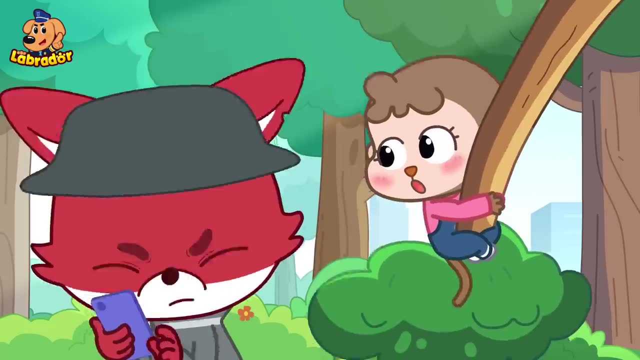 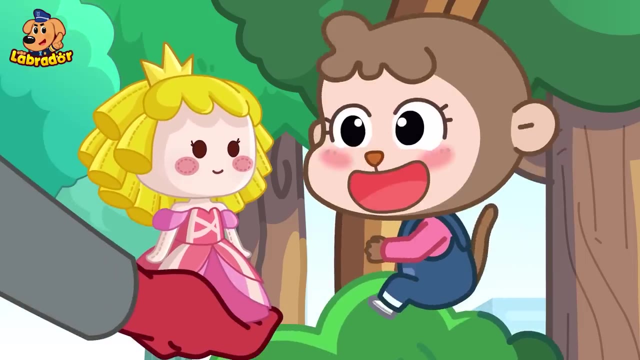 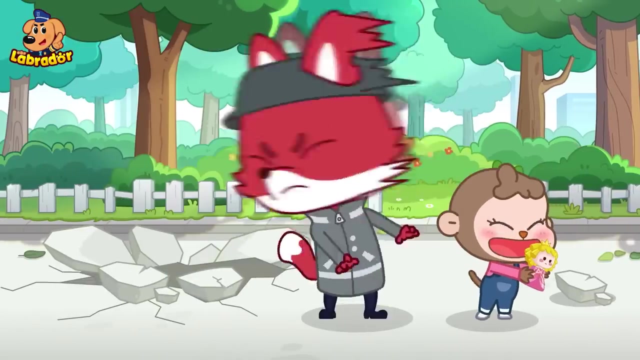 Then did she tell you about what I like too? No, Let me think, Found it. I remember You like climbing trees and you love princesses. Oh, that hurts. Let's go and wait for your mommy over there, Uh-huh. 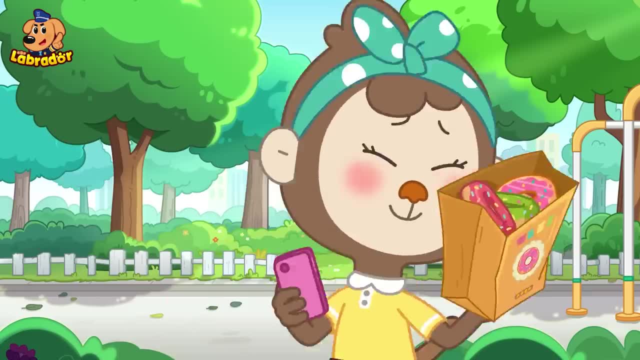 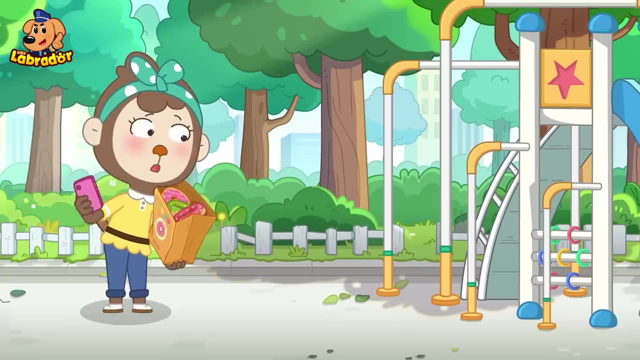 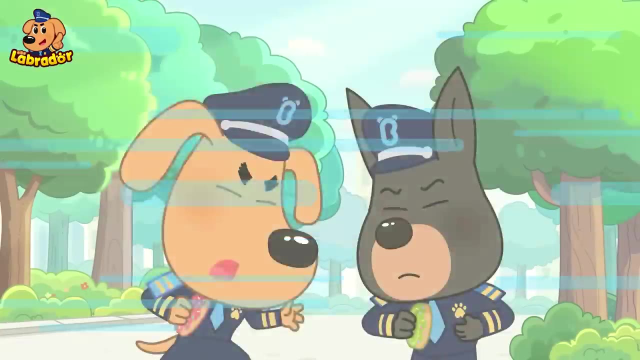 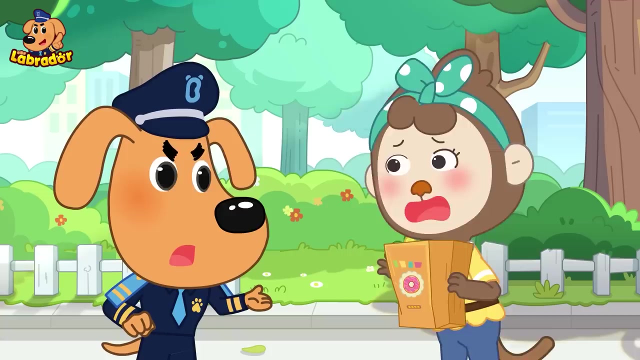 Look, sweetie, Mommy's bought so many donuts. Where did she go, Sweetie? where are you? Let's go, Miss Monkey. what's wrong? Sheriff Labrador, My daughter is missing. She was just here a moment ago. 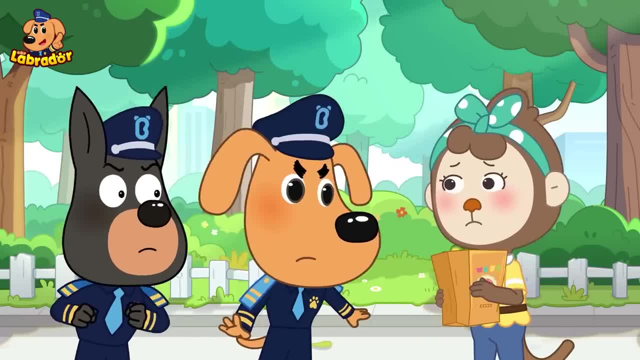 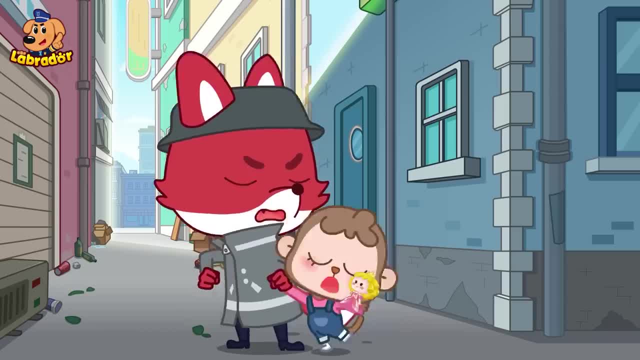 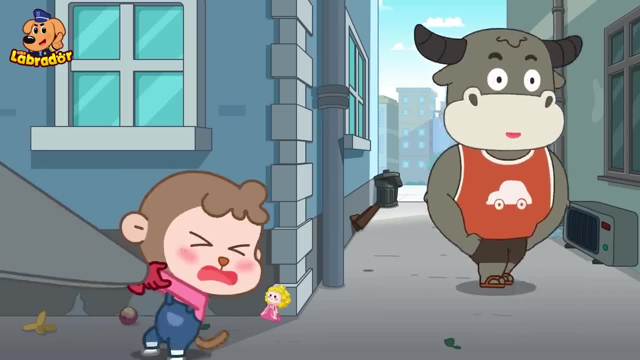 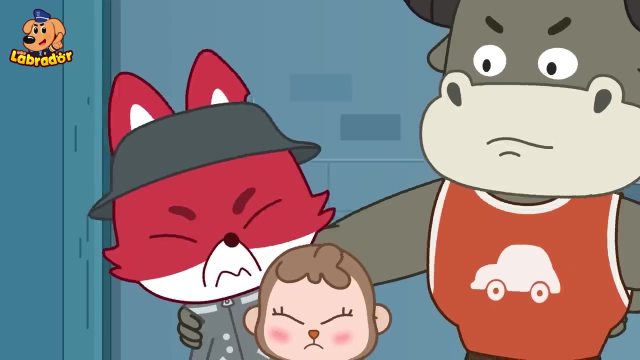 Mr Fox, I think we've gone too far. Be quiet, Just follow me, I don't want to go Hurry. What are you doing? Stop bothering the kid. No, no, I'm just trying to tell her that it's time to go home. 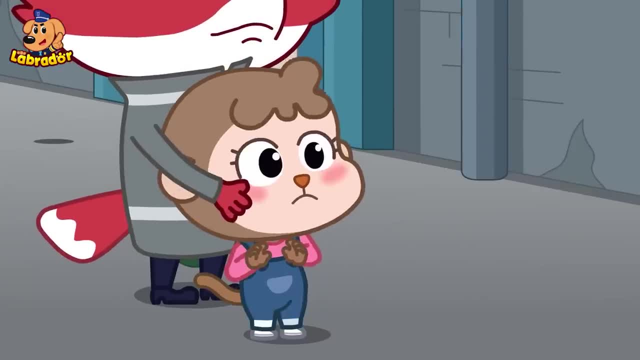 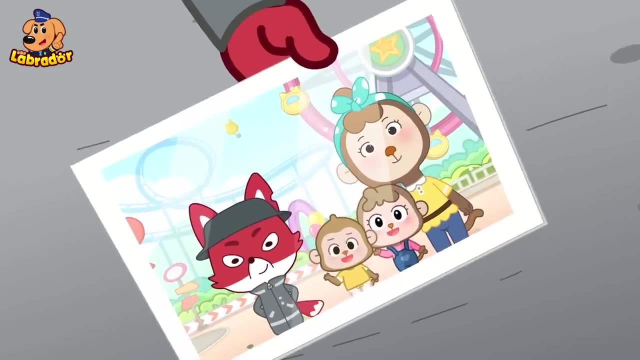 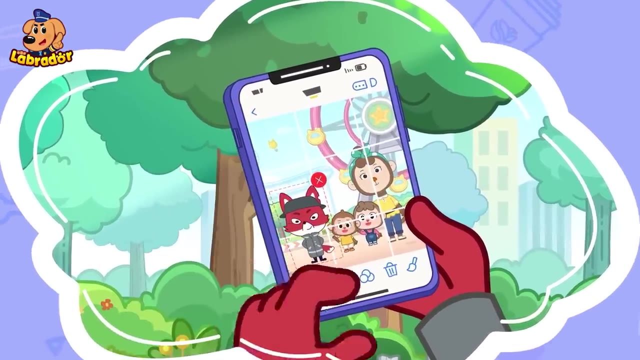 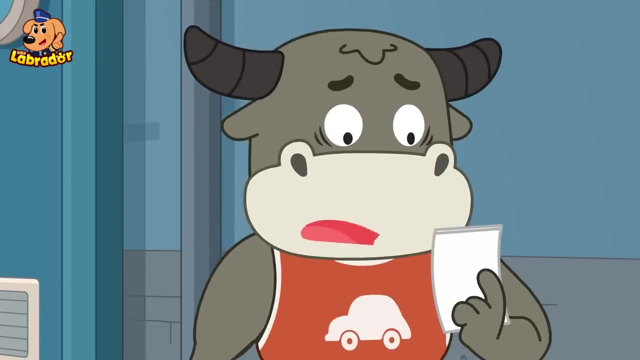 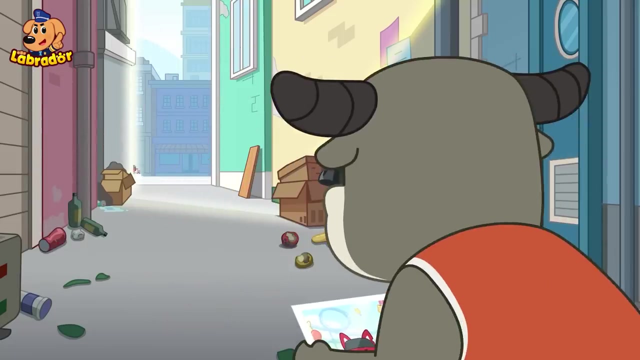 You're a fox and she's a monkey. You don't look like family. I'm a friend of her parents. Look, Good thing I've prepared a picture. Oh, You really are. My little buffalo always keeps me busy too. I need to get out of here. 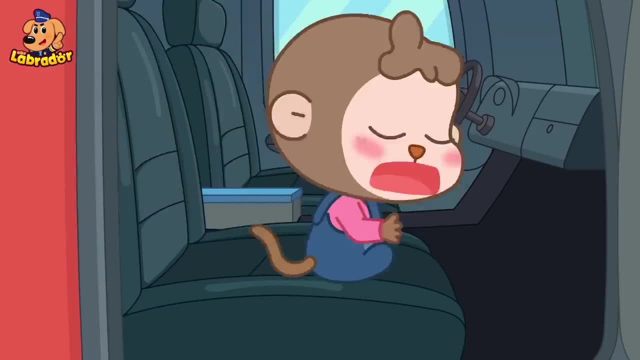 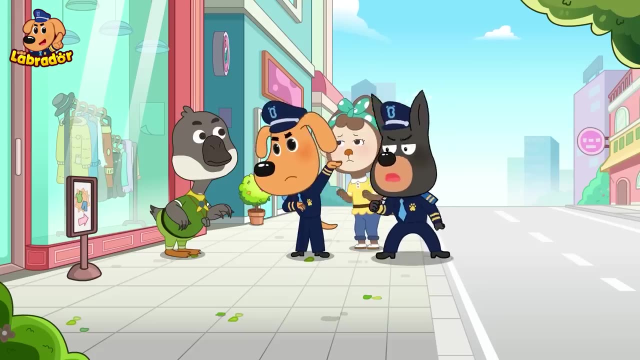 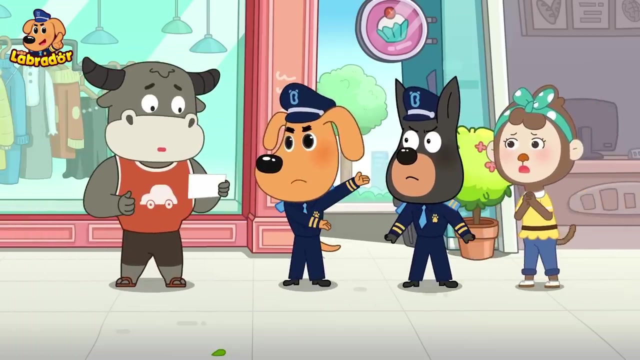 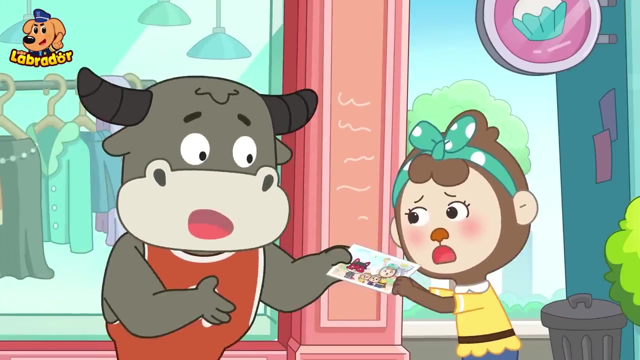 Ouch My car. Have you seen Little Monkey around? Excuse me, have you seen Little Monkey around? Uhyou mean this kid in the picture. How did you get my family picture? That's strange. Why is there a fox here? 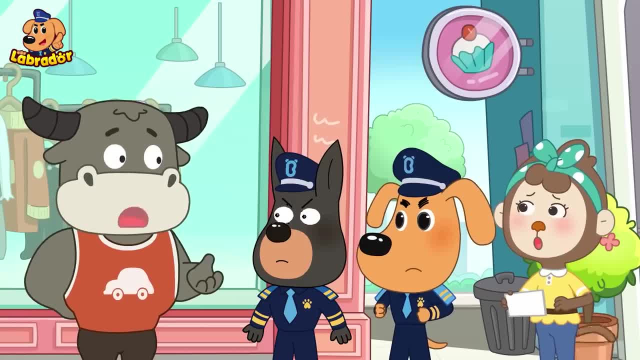 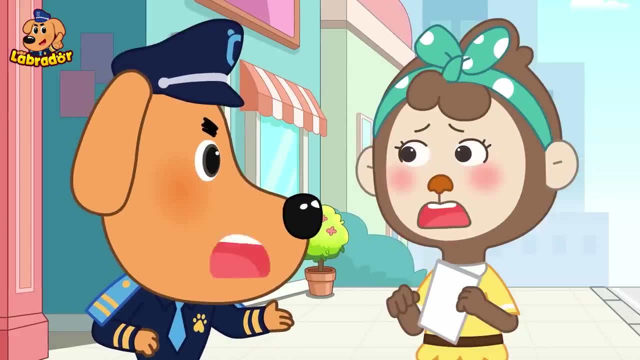 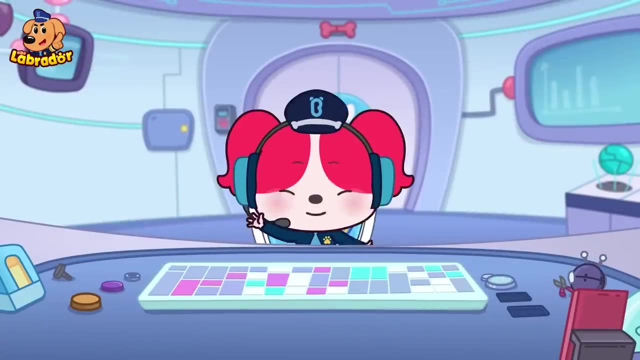 Fox gave me this picture. He said: he's your friend. What? I don't even know him. Hmm, I think Fox used the pictures and information you posted online to take Little Monkey. All crimes leave clues. Oof Hi, This is Papillon. 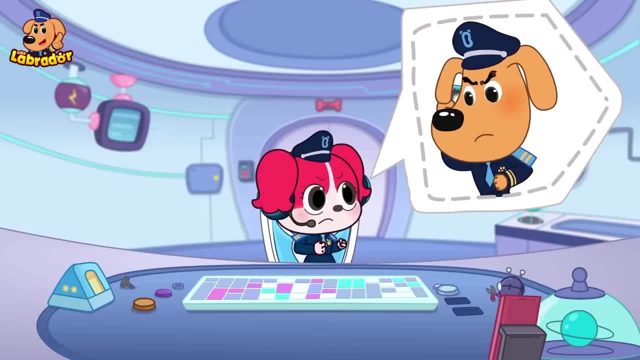 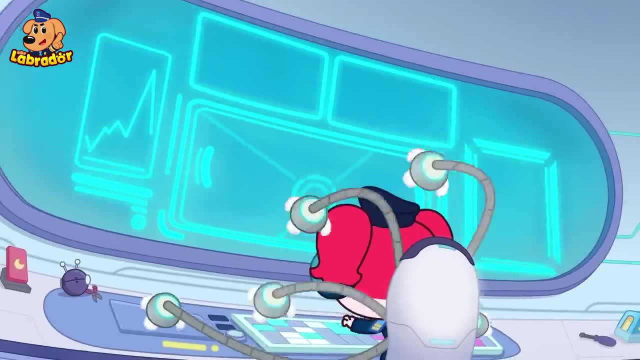 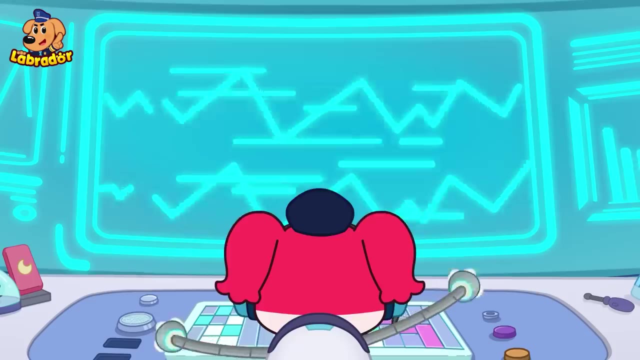 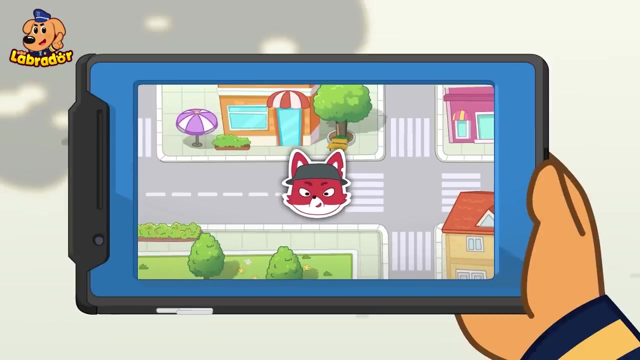 Papillon Fox took Little Monkey. We need your help to find their location. Got it? There's nowhere to run. Show yourself, Fox. Sorry My mistake Sending the location now. Got it This way? Boo, I want to go home.